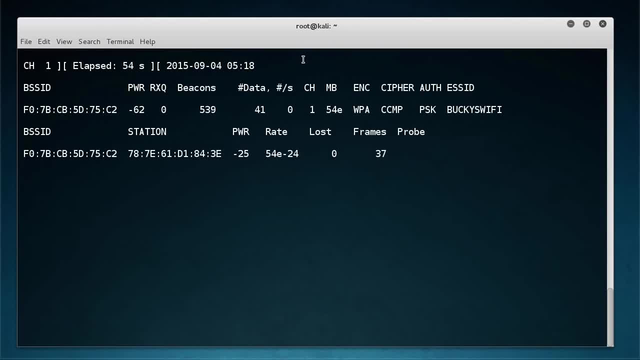 So there you go. I started listening for traffic. So what we need to do right now is we need to wait until a handshake takes place. Now, the handshake, like we saw in the last video, that's the authentication process, basically a device proving to the access point that it does know the password. 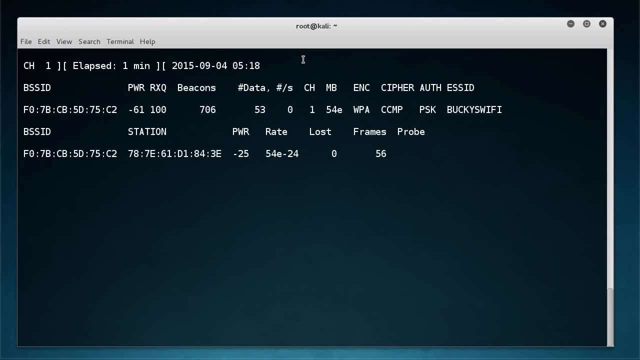 Now, whenever this happens, we can look at that traffic, pull all of the useful data that we need out of it and plug it into the formula where we can perform our dictionary attack. So we pretty much need for some legit person to log into the networks. 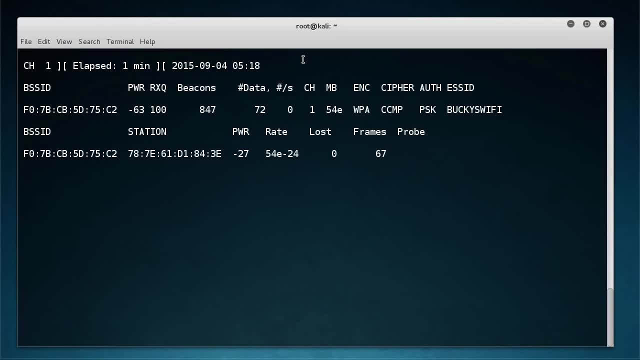 like an employee, a teacher, whatever. Now, if you're at like a huge office building or like a university or something people are going to be like, we're going to be logging into this network all the time. However, if you're a smaller establishment or maybe just like someone's home, 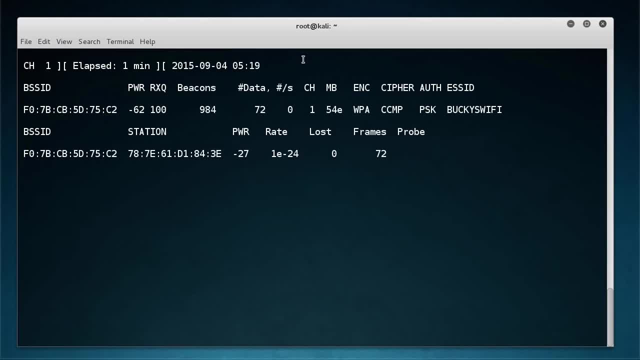 it may take a while for someone to actually- you know- log in to the network. So if you don't want to wait, what you can actually do is find someone that's already connected and just send them a deauthentication packet. So then you kick them off and they're going to log back in right there. 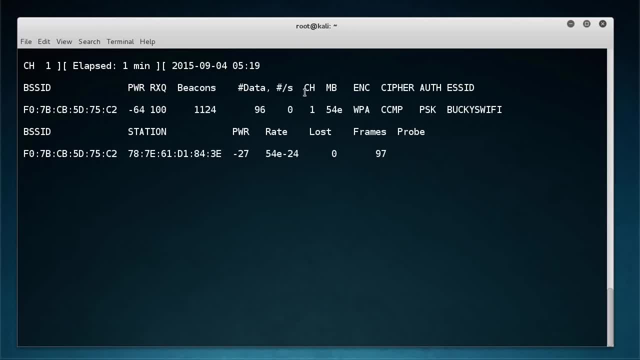 So that's a cool little trick, But take note of this: I'm picking up my tablet and I'm not connected yet And I'm about to type in the password and log in And watch what happens in this top right area As soon as we capture that authentication which is called a handshake. 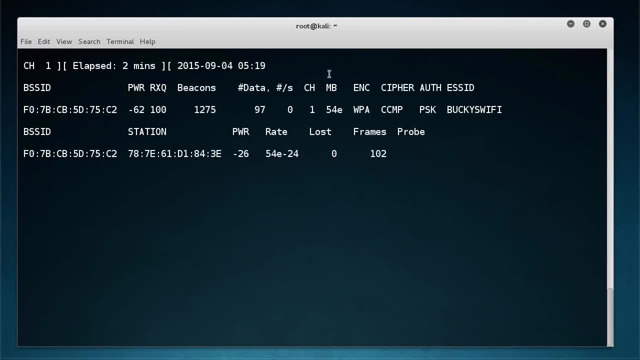 it's going to give us a little indicator. So it's really awesome. You don't have to like: guess, did I get one yet? Did I get one? It's going to tell you. So I picked up my tablet and we'll just pretend like I'm a teacher. 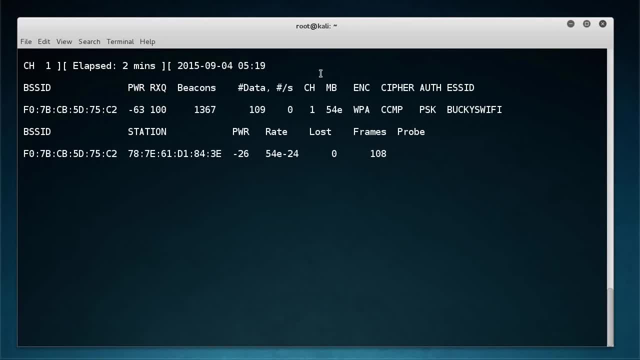 like someone legit that knows the password. Go to my settings, choose this network And then let me type in bacon123.. Now I'm about to hit connect And again keep your eye on that and check it out. So it says WPA handshake. 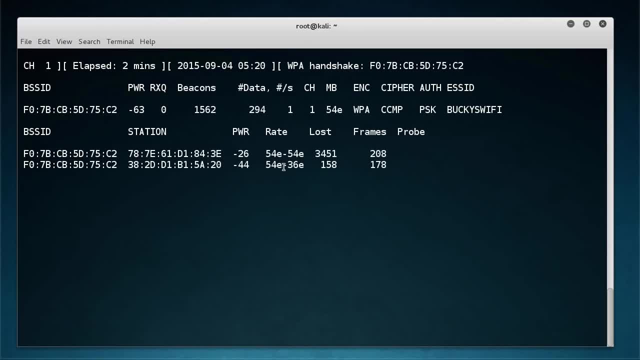 And this means that we did capture one. So now I can just hold down control C to stop that We got the information that we needed. Now, just so I can show you guys real quick. if I go to my captures right now, you see that this is the data we collected and all these different formats. 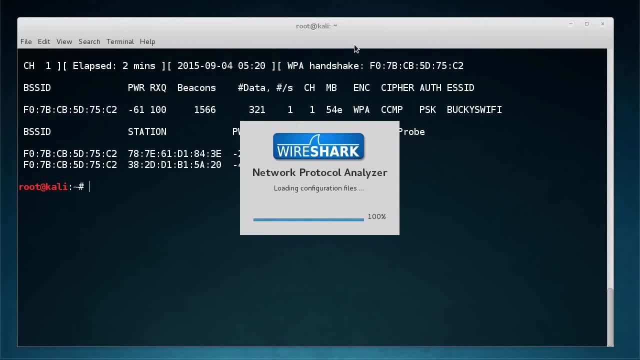 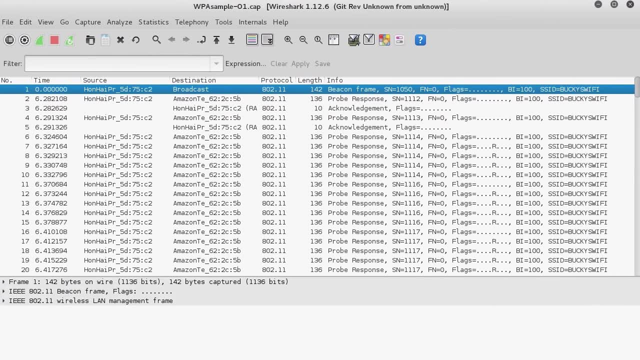 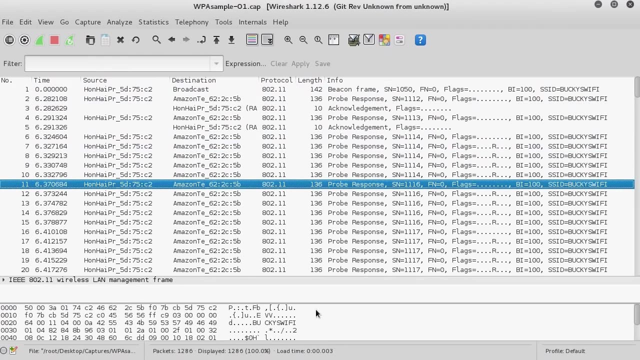 I'm going to right click this and open in Wireshark And check it out. rearrange until you guys can see. All right, So this is all the packets that we caught And if we try to read any of these, not going to be very successful. 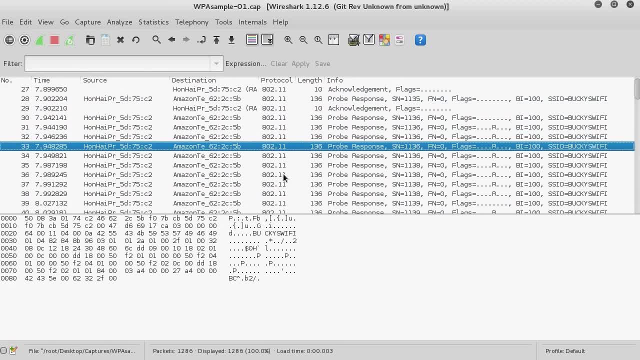 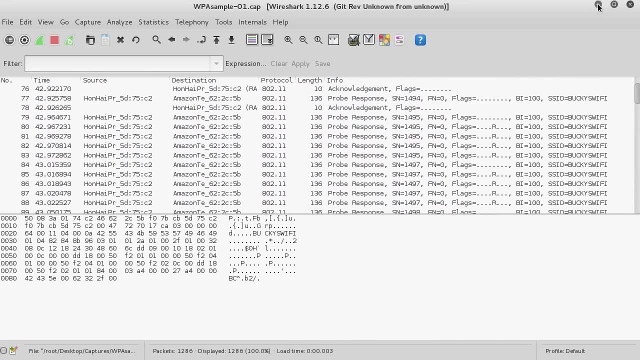 So it's pretty obvious that right now, even though we can look at some data, it is all encrypted. This is useless to us. So what we're about to do next is we are going to loop through the passwords And we're going to plug them each into. 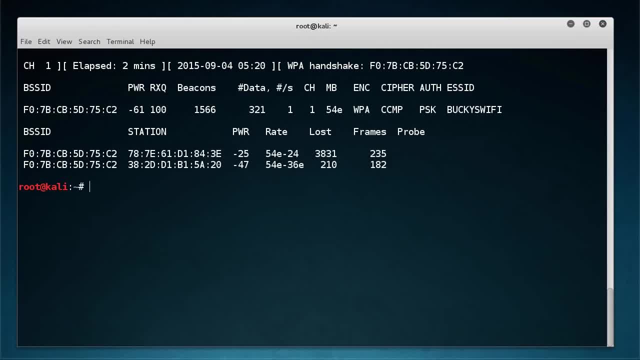 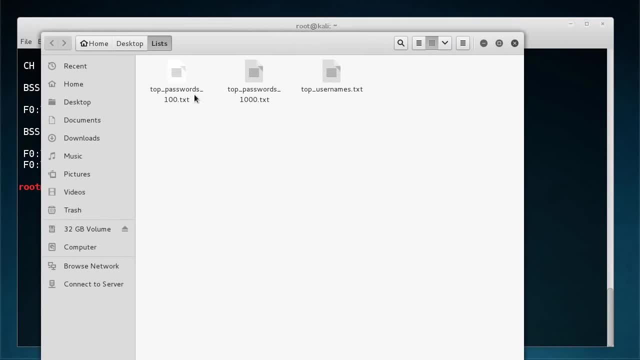 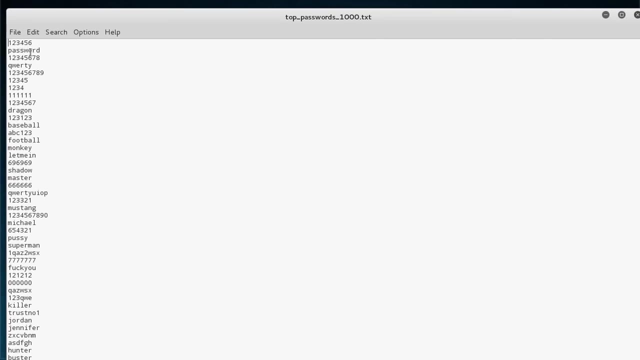 The formula and we're going to see what one works. So what you need is actually a list of passwords, and they are all over the internet. I'm going to show you the one that I got. I actually got this off of GitHub, So these are just the top 1,000 common ones: one, two, three. password: one two, three. 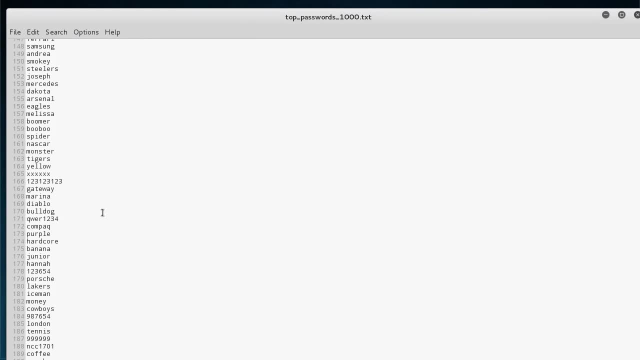 four, yada, yada, yada. And let me show you guys something. So I put my password online. Where are you at? Where are you at? All right, That's my password right here. So I was going to try all of these. 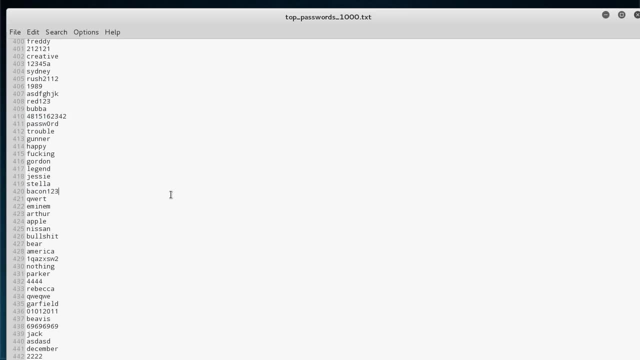 And then, whenever it gets to mine bacon one, two, three, it's going to go dun, dun, dun. Well, it's not actually going to make that sound, but it's going to be thinking about it. It's going to be like, hey, I found the right password. 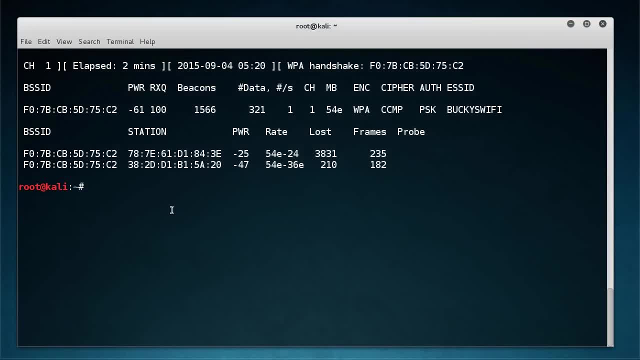 I found something that works And this is incredibly easy. So for this we're going to be using a tool called Aircrack NG. Now I'm going to talk to you guys about a little rant. The entire suite of tools, like the collection of tools that we're using for Wi-Fi. 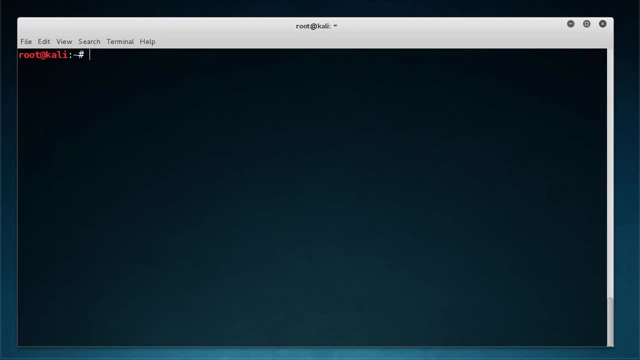 It's called Aircrack, And one of the tools in here is actually called Aircrack NG. So the name Aircrack isn't the name of the collection, It's also a name of a tool. So it gets kind of confusing, but don't let it throw you. 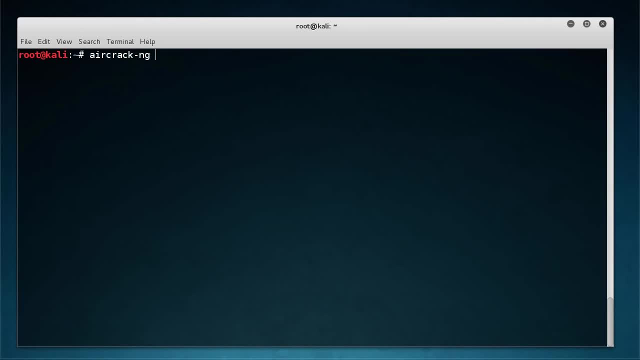 So Aircrack NG- that's what we're going to do- to crack the password. And then it takes two pieces of information. The first one is the capture file, the one that we just opened in all Wireshark And mine is in desktop captures. 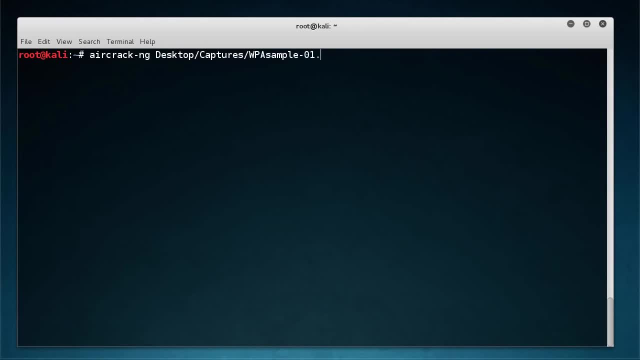 And it was called WPACAP. Now the next thing it needs is: all right, what are all the passwords that you want me to try? And that was that file I just showed you guys And it was desktop list And I believe it was called: no top passwords and 1000. 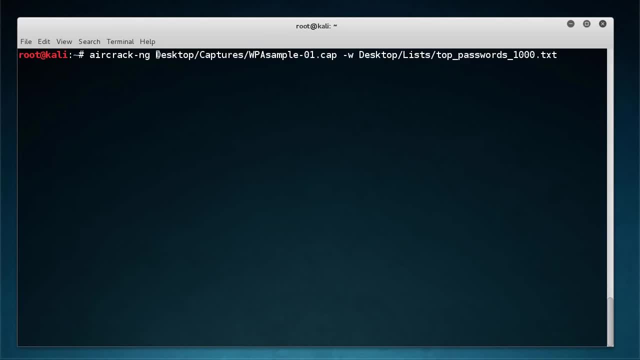 So, again, in order to find the right password, all you need is a capture file that has the handshake in it And a list of possible passwords. Now I'm going to hit enter And it's going to start looping through those. And how quick did that take? 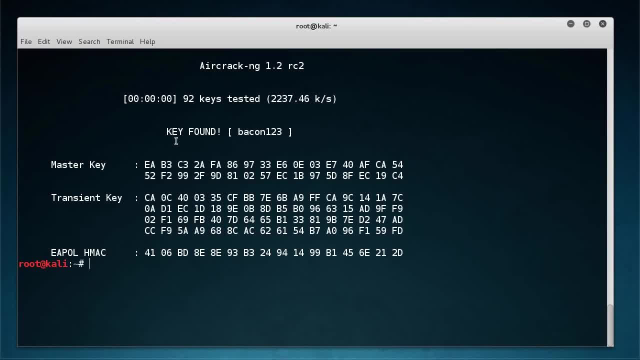 Like a second, a second and a half maybe, And what it says is: okay, I found your key, bacon123.. I mean in a blink of an eye, And, by the way, I just want to say that it doesn't usually take that quick. 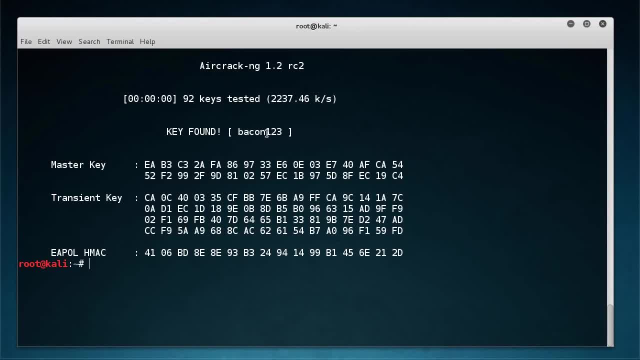 Sometimes people have like millions and millions of passwords. Sometimes it can take quite a long time, But I mean, this is a computer. It just ran through 400 potential options in like half a second. And I mean, if you ever looked at anyone's password on their Wi-Fi, they're usually not. 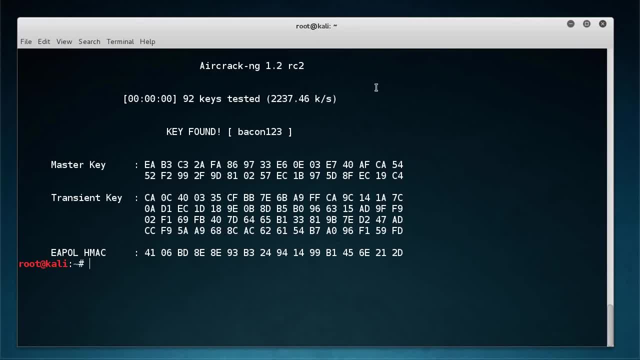 that complex, like the majority of people, So that is how you perform that. Now, what I'm going to do, now that we have the password, is: we now have all the pieces that we need. Not only can we log in to the network just using this password, but we can also start. 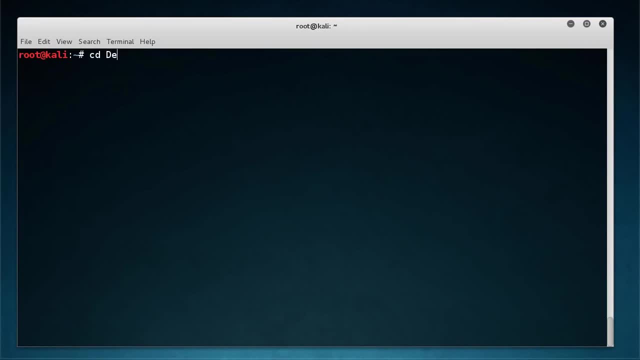 decrypting All of that information. So now let me move over to my captures file, And what we can do here is we can run a tool called airdecapng, And this is a tool that you use to actually decrypt those packets. 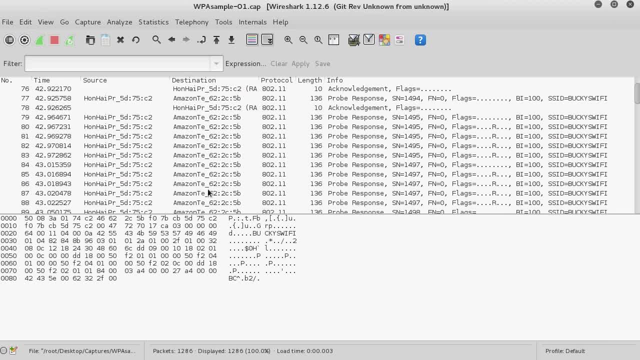 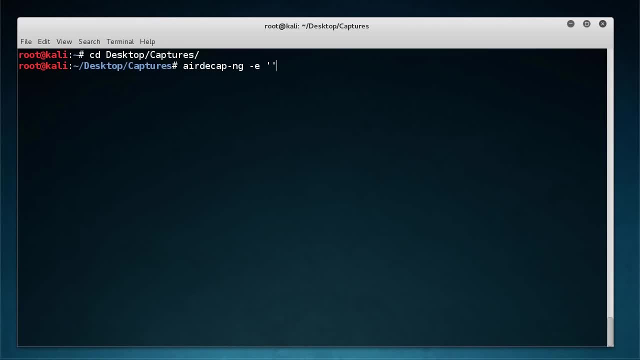 So, now that we have all the pieces, what we can do is we can start looking through these packets and decrypting them. Pretty awesome. So the formula takes a couple pieces and we already have all of them. The first thing is: What's the name of the network?